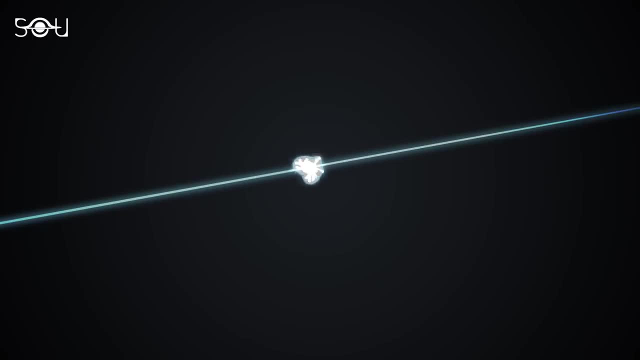 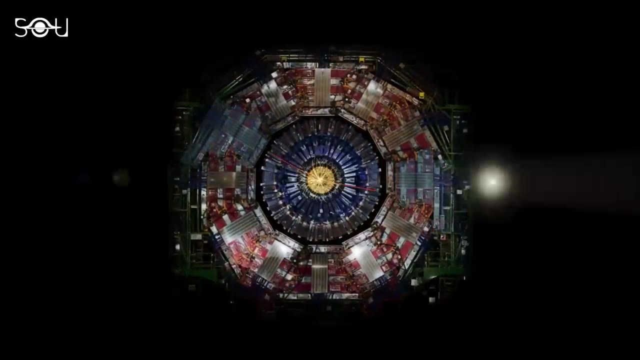 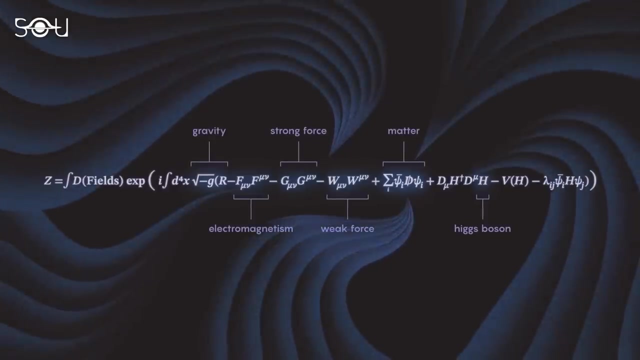 Scientists have observed a puzzling event related to the Higgs boson, which shows our understanding of the particle may not be correct. They've observed an unexpected decay of the exotic particle that's far beyond the accepted realms of the standard model of physics. These unexpected findings challenge the predictions of the standard model. 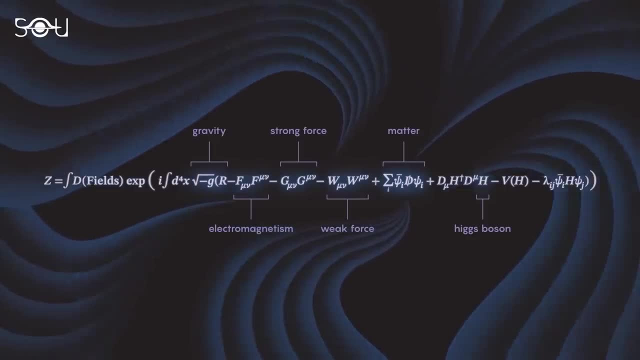 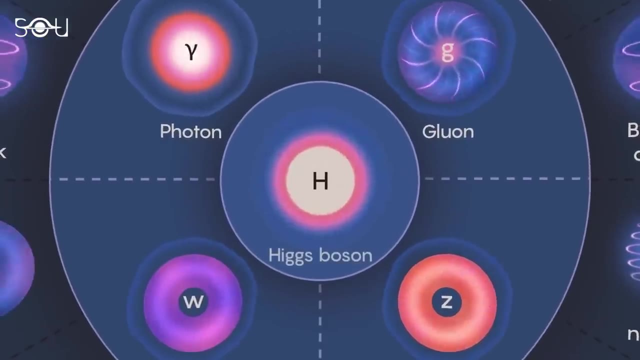 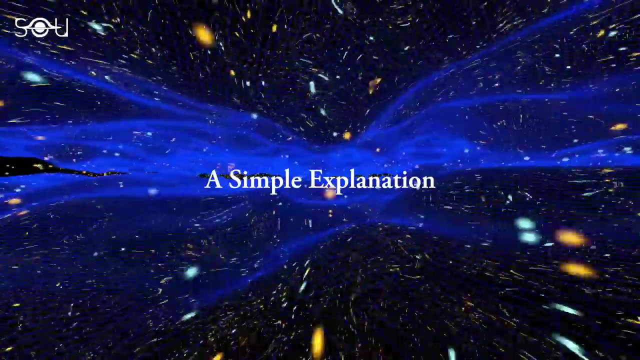 and indicate the possibility of new physics at play. To understand what's been observed, let me briefly explain the concept of Higgs boson and the Higgs mechanism using a daily life analogy. Picture the universe as a vast swimming pool filled not with water but an invisible substance called the Higgs field. Now imagine. 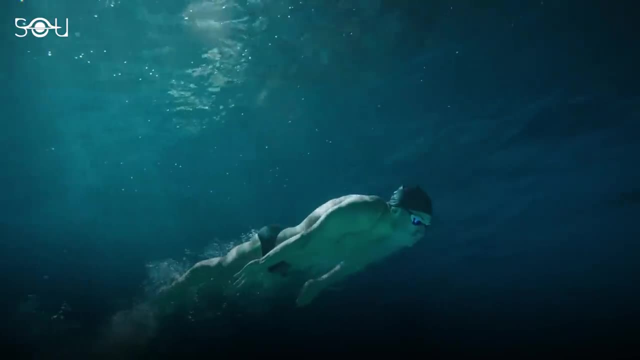 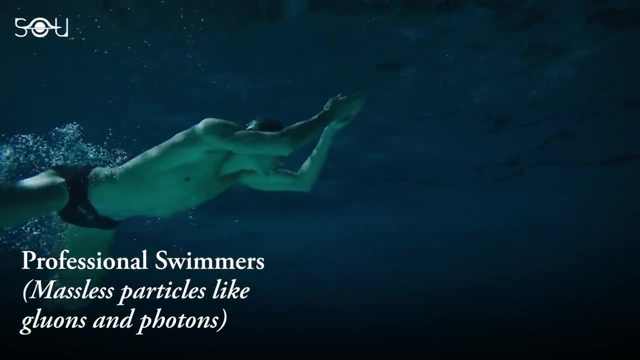 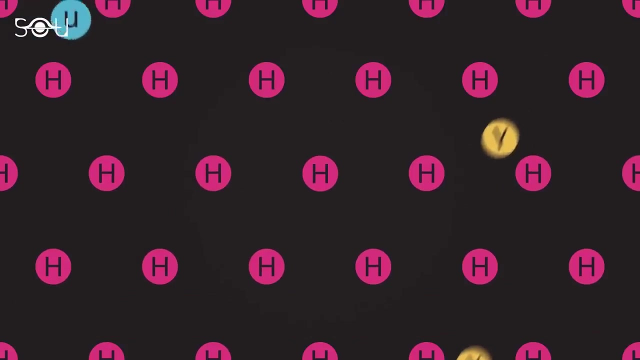 different types of swimmers in this pool. The first swimmer is a professional streamlined inefficient. As they swim, they slice through the water effortlessly, barely interacting. This is similar to particles like photons, which don't interact with the Higgs field and hence 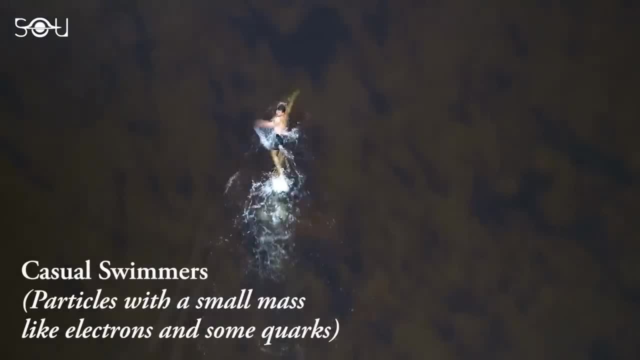 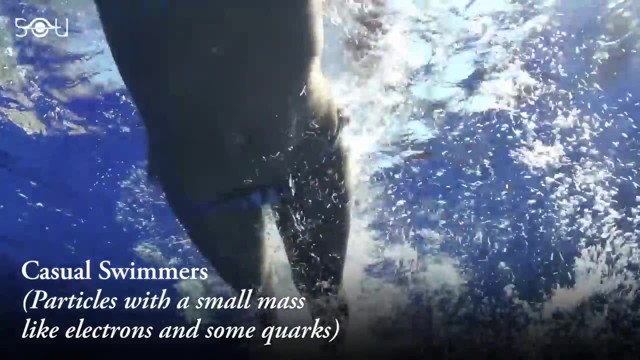 are massless. Next, think about a casual swimmer, maybe someone who doesn't swim often. They can swim, but they create a lot of splashes and waves and they find it harder to move through the water. These swimmers are like particles such as. 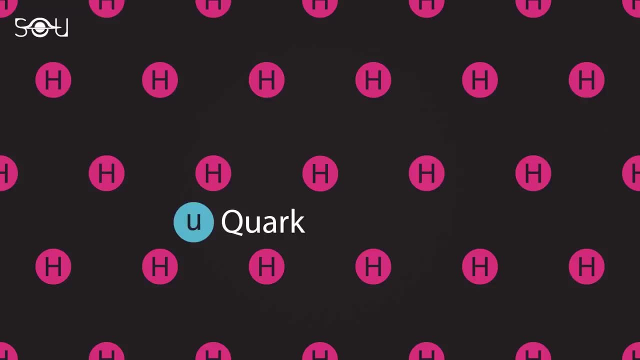 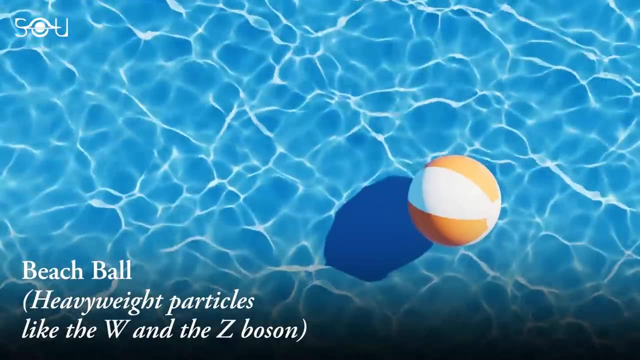 electrons and quarks. They interact with the Higgs field, which is why they have mass. Now imagine if the Higgs field had a mass that was equal to the mass of the Higgs field. Imagine if the Higgs field had an inflatable beach ball in the pool. This ball can't move. 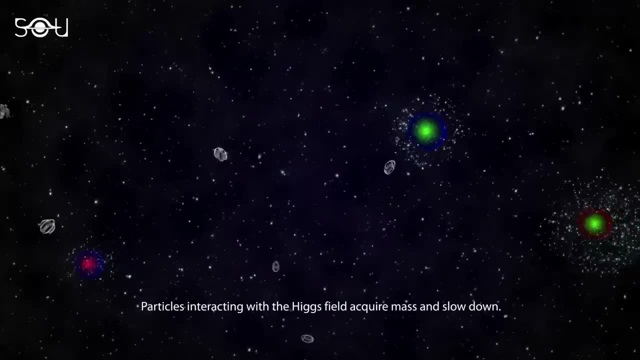 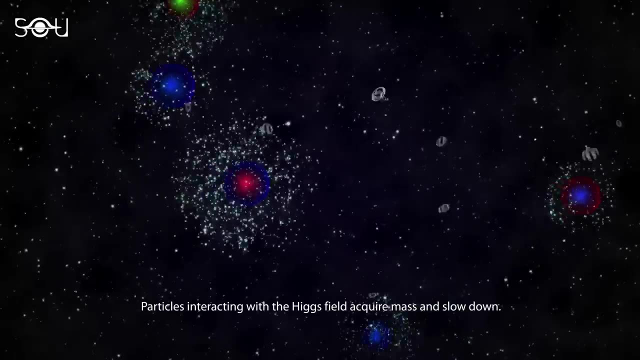 on its own and it takes some effort to push it around. So we can think of the beach ball as representing heavier particles like the W and Z bosons. They interact with the Higgs field a lot, which is why they have a lot of mass. Lastly, imagine the waves that move across. 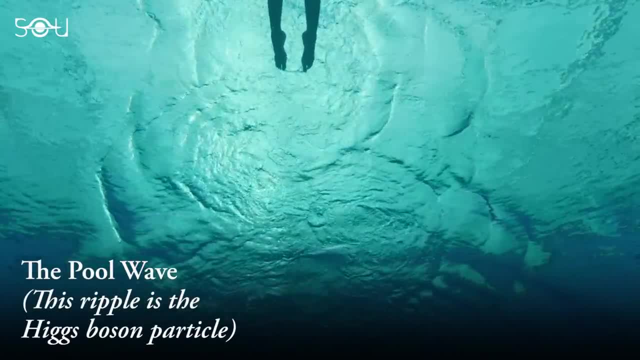 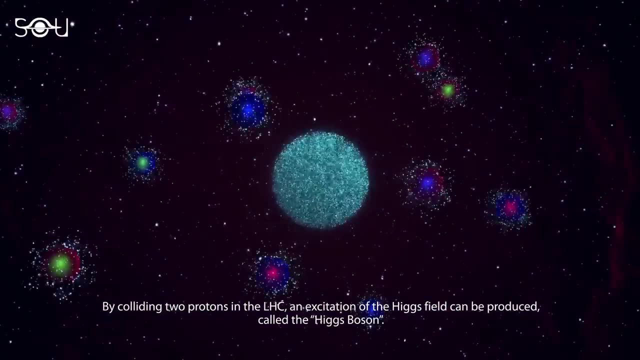 the surface of the pool when the swimmers move. These waves are like the Higgs boson. When a particle interacts with the Higgs field, it can create a disturbance or a ripple like a wave in our pool. That's the Higgs boson. 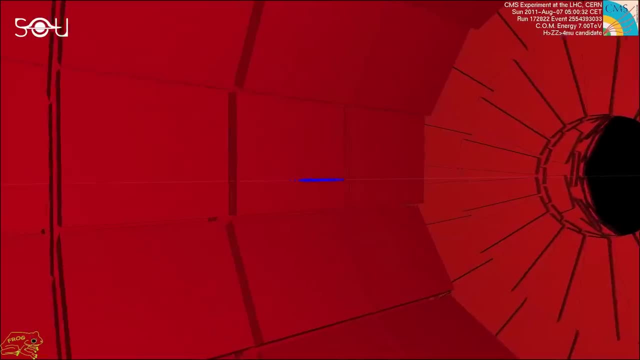 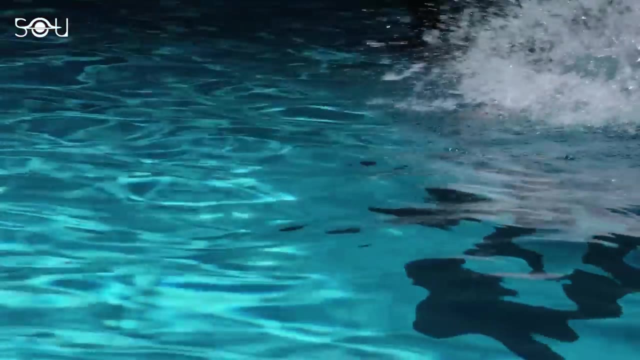 a quantum excitation of the Higgs field. When we discovered the Higgs boson at the Large Hadron Collider, it was like seeing those waves in the pool. It was confirmation that there must be swimmers or particles moving and interacting with the pool or the Higgs field. 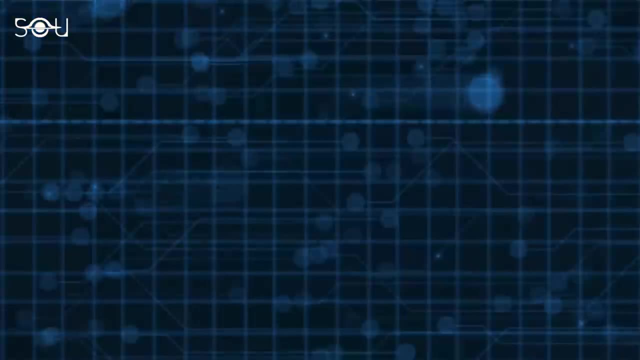 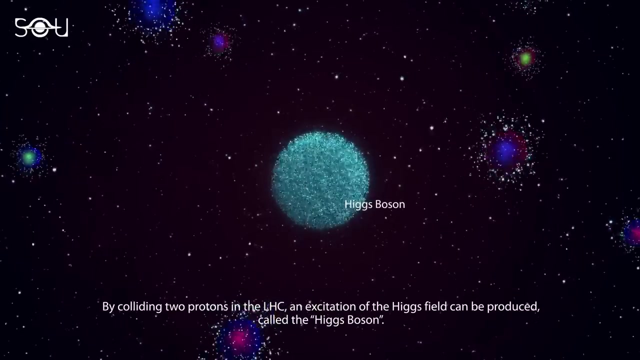 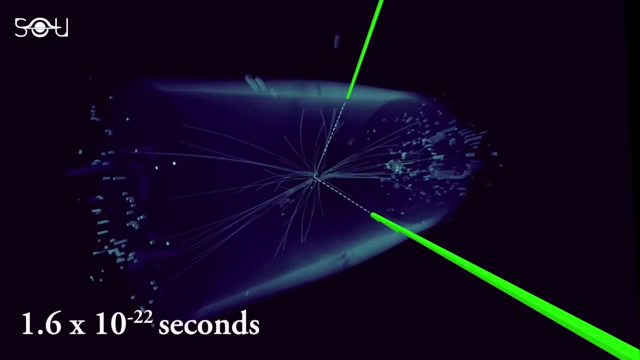 Now the problem is that the Higgs boson doesn't stick around for long Once it's created in particle collisions. the famed particle lives for a mere less than a trillionth of a billionth of a second, or more precisely, 1.6 into 10 raised to the power. 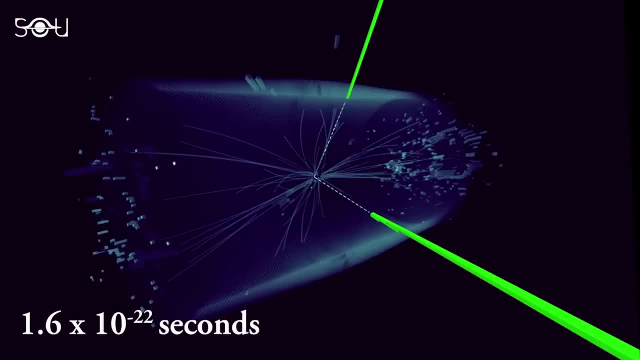 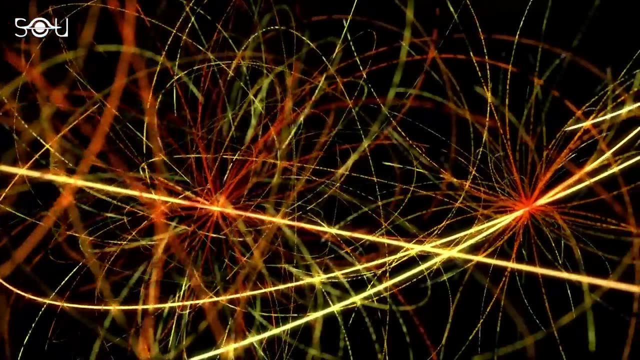 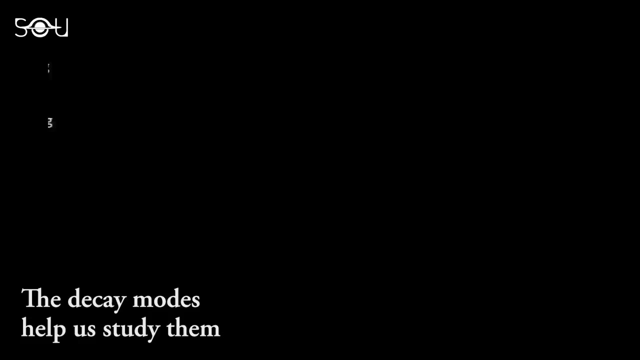 minus 22 seconds. This makes it very challenging to study the particle. It's like the particle is created and destroyed in an instant. So one way that physicists study the properties of such short-lived particles is through their decay modes. This decay can happen in several ways or modes, and which one occurs depends on the specifics of 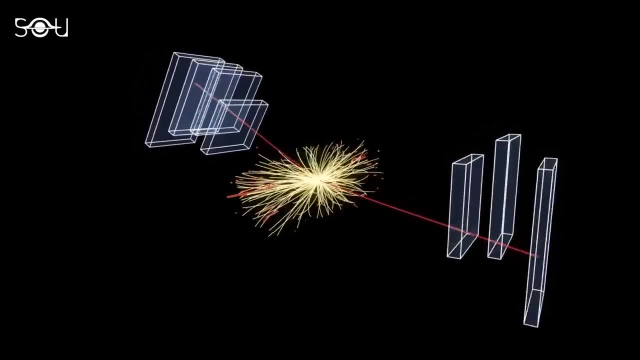 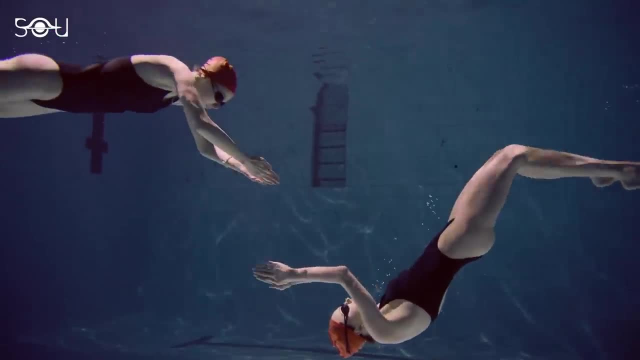 the conditions And the unusual event related to the Higgs boson involves its decay into another set of particles. Let's get back to our swimming pool analogy. Let's say our swimming pool wave or the Higgs boson becomes too big to sustain What happens? 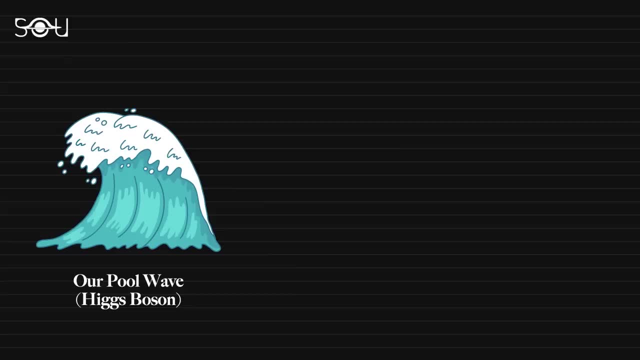 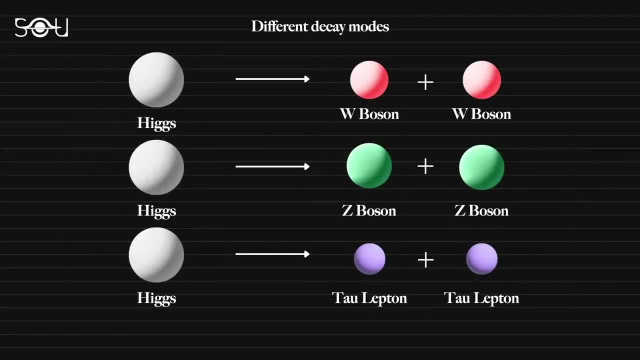 next It needs to settle down right. And how does it do that? It breaks up into smaller ripples or waves. Now imagine that these smaller waves represent other particles, Depending on the initial size and energy of our big wave or the Higgs boson. 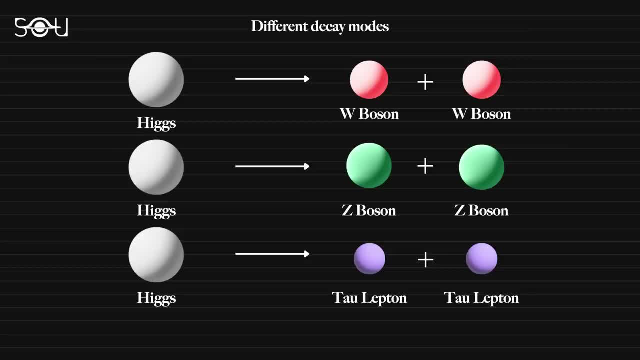 it could break into a pair of smaller identical waves, like a pair of W bosons, Z bosons or Tau leptons. It could even create a mix of waves and tiny bubbles, like a pair of leptons and photons. It could even create a mix of waves and tiny bubbles, like a pair of leptons and photons. 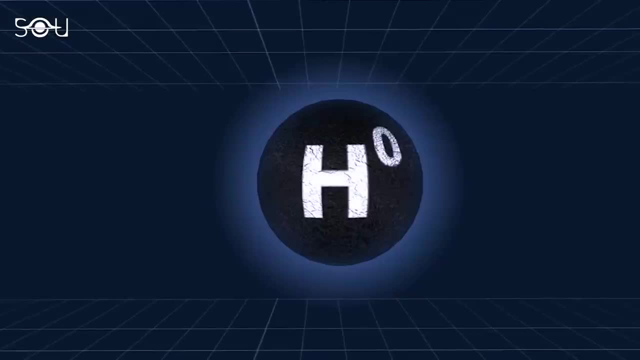 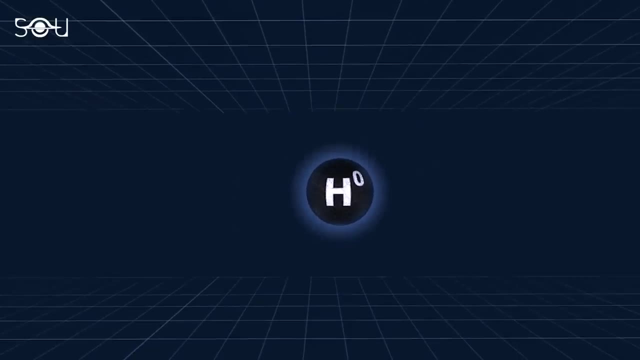 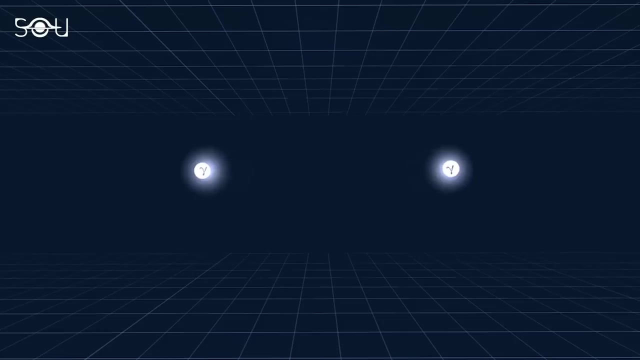 Now this is where things become tricky. The decay process of the Higgs boson into two photons is not a straightforward one. Instead, it involves a convoluted mechanism, known as a loop, wherein virtual particles temporarily appear and disappear. These virtual particles can 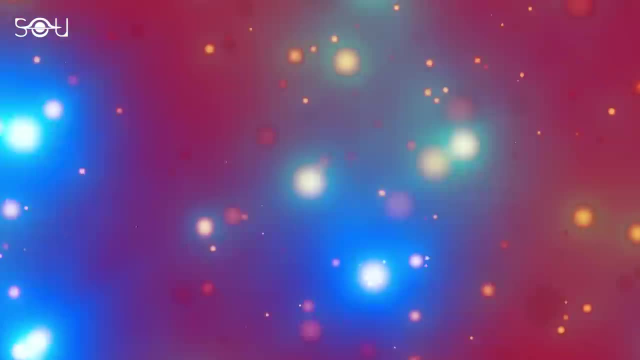 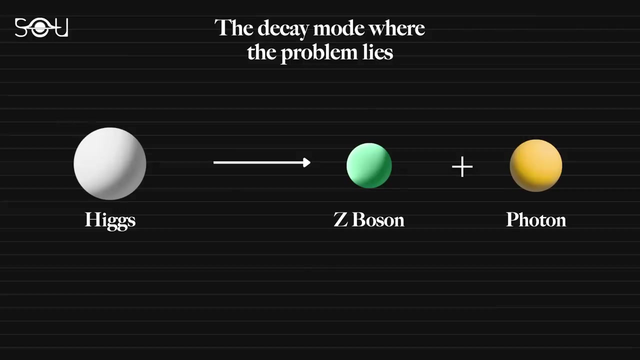 include hypothetical particles that have yet to be observed, making their direct detection impossible. Interestingly, this process is not limited to the decay into two photons. It also applies to the decay of the Higgs boson into a photon and a Z boson, which is the focus. 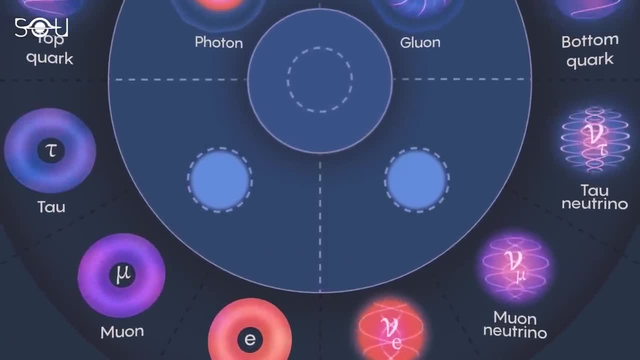 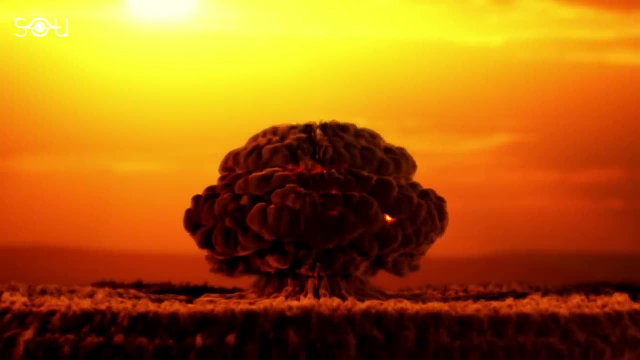 of the new study. The Z boson is the heavyweight of the standard model, an elementary particle that, along with the W boson, is the carrier of the weak nuclear force At the Large Hadron Collider. researchers sought to investigate this rare decay process. 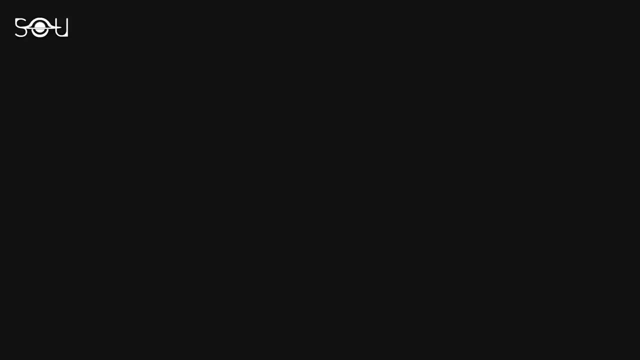 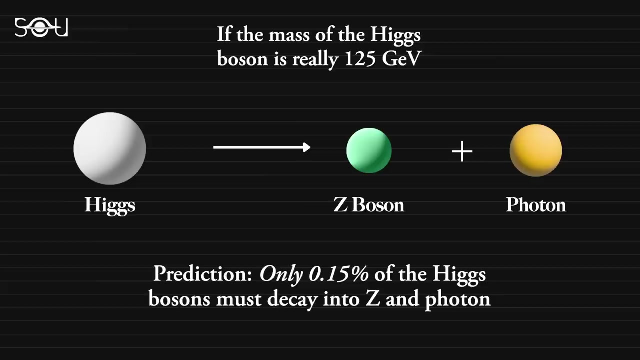 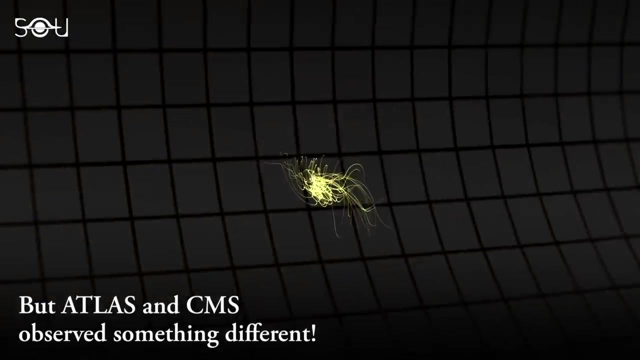 According to the predictions of the standard model of particle physics, only a tiny fraction, or 0.15 percent, of Higgs bosons should decay into a Z boson and a photon. However, the experimental data gathered from proton-proton collisions conducted at the 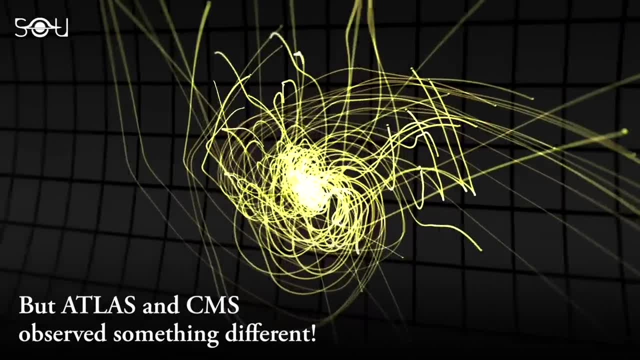 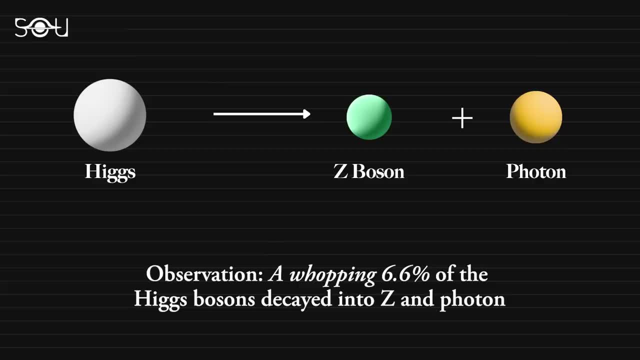 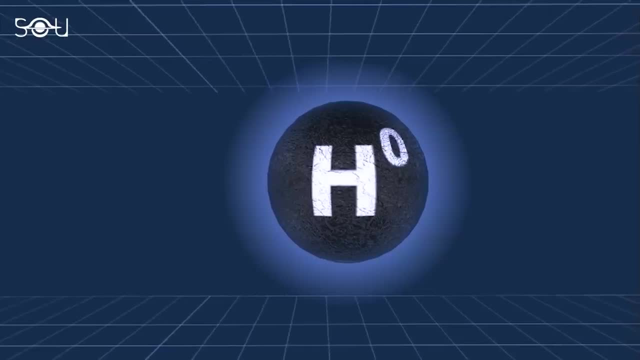 ATLAS and CMS detectors between 2015 and 2018 paints a different picture. Surprisingly, the data reveals that this decay is occurring in around 6.6 percent of cases. a significant deviation from the expected value. The Higgs boson was identified by observing its subsequent decay into pairs of electrons. 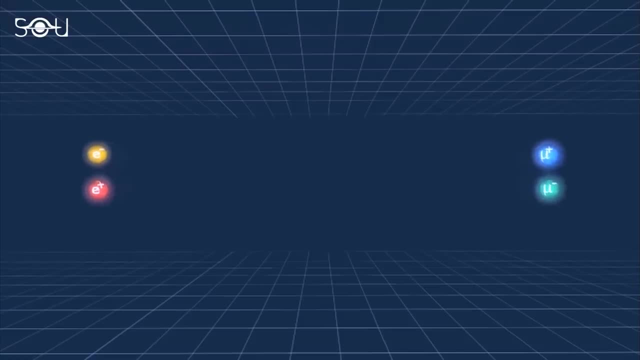 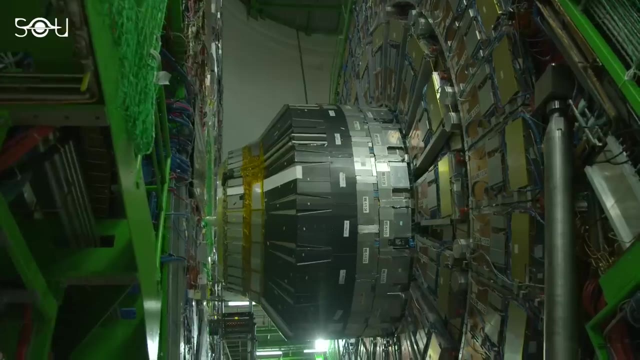 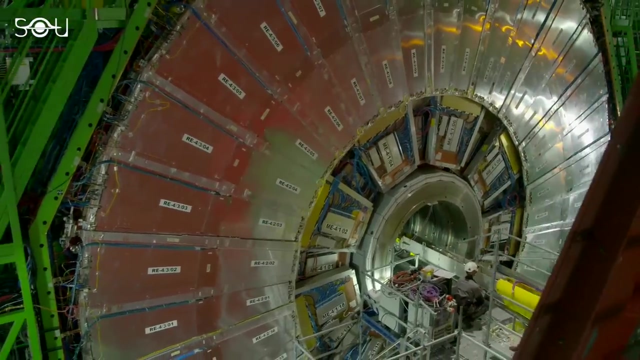 or muons, and the frequency of these Z boson decays was found to be approximately 6.6 percent. ATLAS and CMS, the two key experiments at the Large Hadron Collider, employed strategic approaches to maximize the sensitivity in detecting the decay of the Higgs boson into 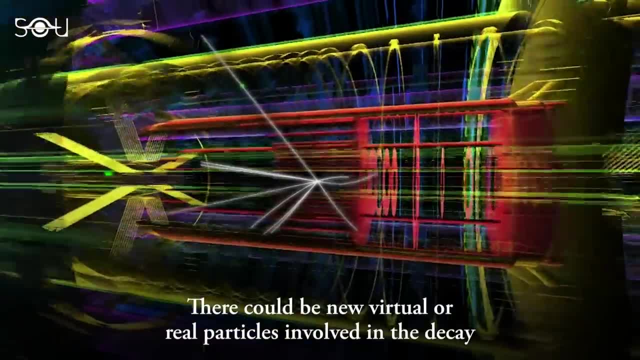 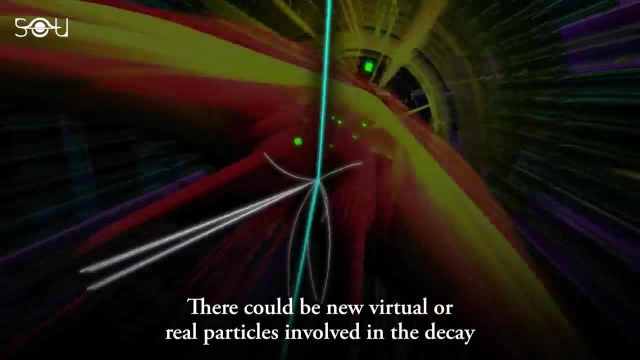 a Z boson and a photon. By focusing on the most common modes of Higgs boson production, utilizing advanced machine learning techniques, they were able to distinguish between signal and background events effectively. As a result, they obtained the first evidence of this decay. 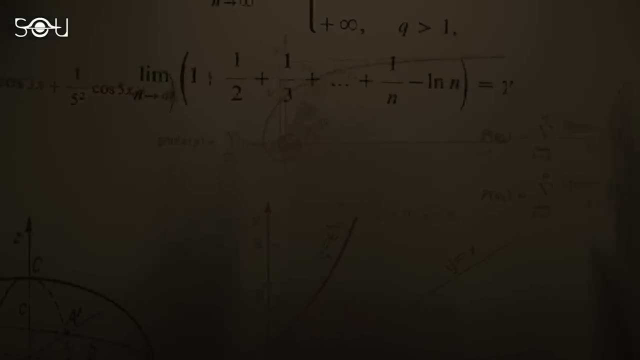 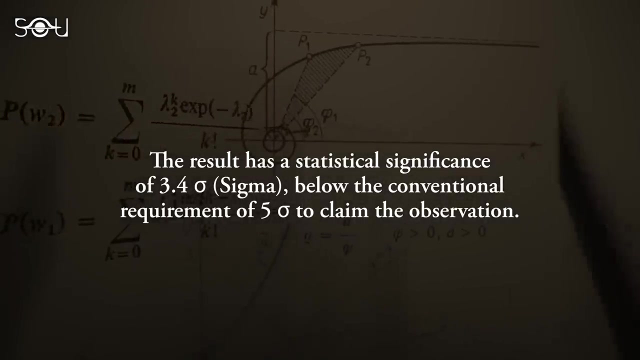 process. However, it's important to note that the statistical significance of the observations stands at 3.4 standard deviations, slightly below the conventional threshold of 5 standard deviations required to claim a definitive observation. This indicates a small possibility of the findings being a chance occurrence. 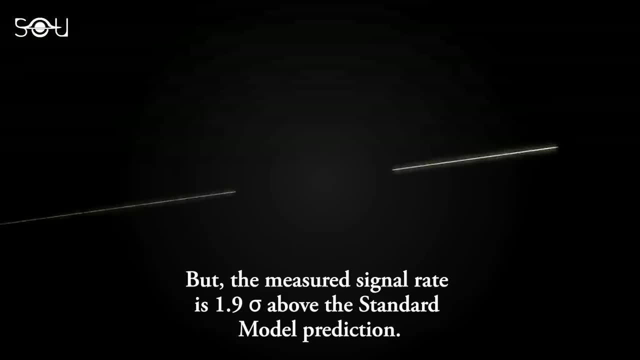 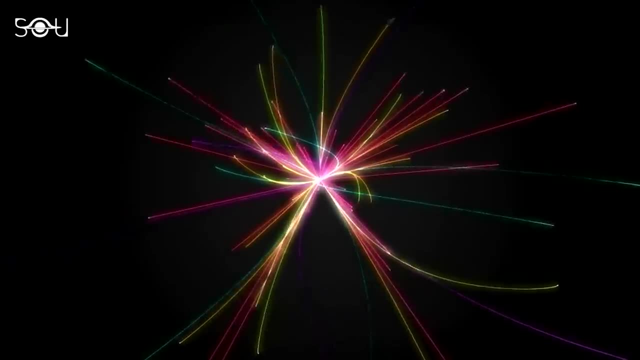 Nonetheless, the measured signal rate deviates from the predictions of the standard model by 1.9 standard deviations, which makes it a notable result worthy of consideration. The Higgs boson has long been regarded as a cornerstone of the standard model of particle.